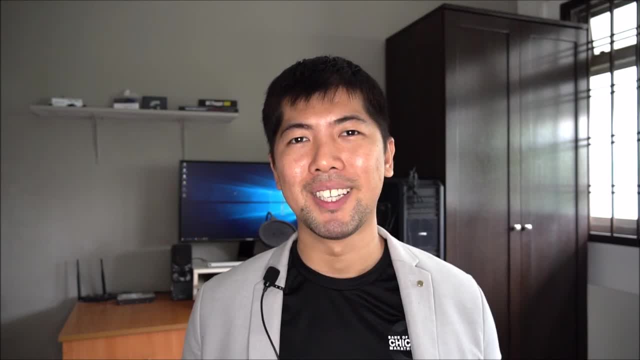 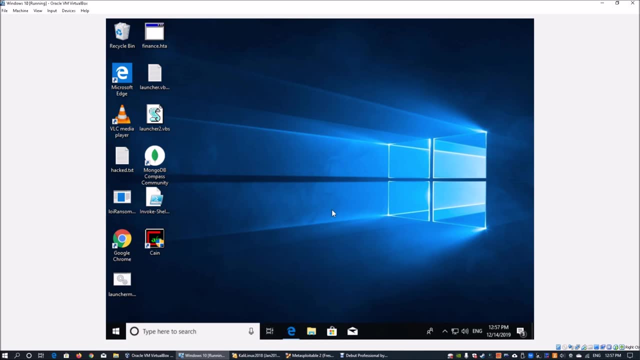 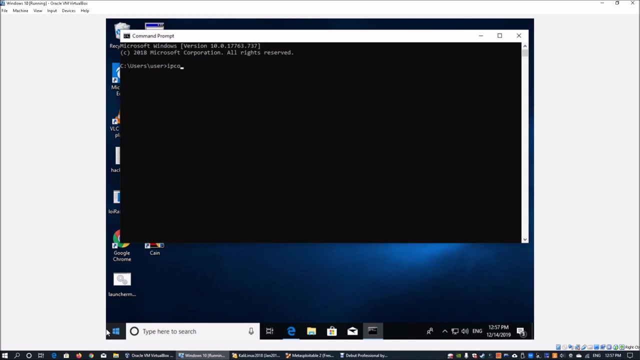 perform the attack. So let's get started. So here I got VirtualBox running and we got Windows 10 over here on one of the virtual machines. So I can enter CMD and we can enter the IP config to see the IP address of the target. 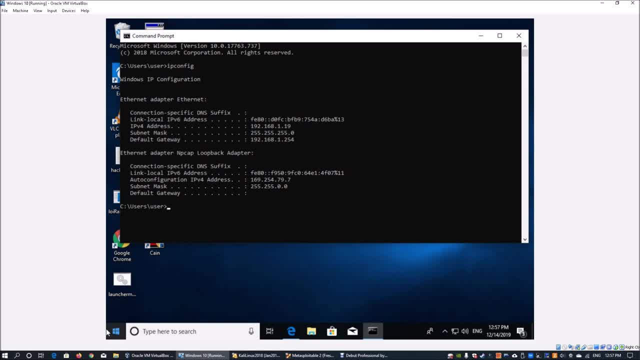 machine. So Windows 10 is going to be the victim machine. so whatever browsing information it is going to access into a server, we'll be able to see it and be able to take note of the user information that we're going to be accessing into a server. So we're going to be able to see it. 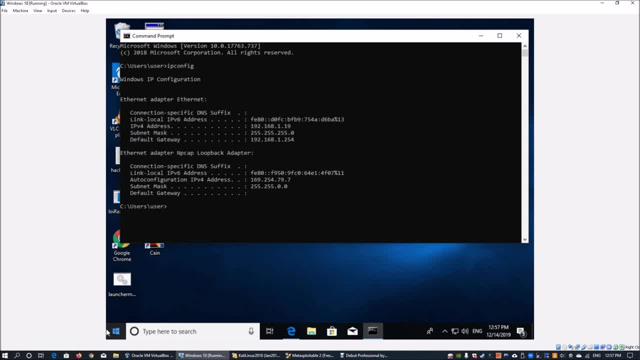 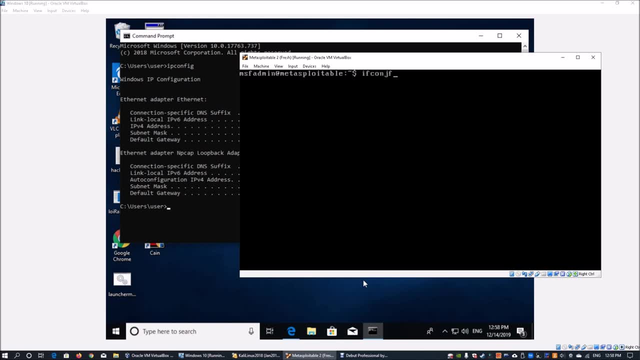 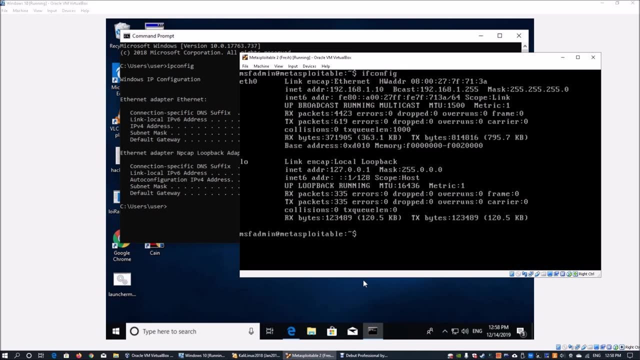 names, passwords, browsing and so on. So, moving forward, we got the server running. So here I have man-exploitable and I can enter ifconfig. So ifconfig would actually tell us the IP address of 192.168.1.10.. So this is the target server. So we got a target victim and we got a target. 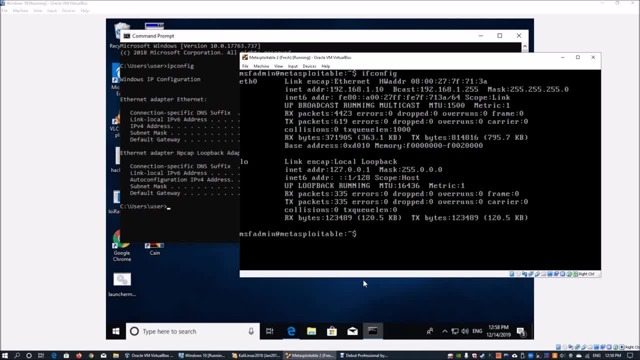 server And then from here on we will be able to actually conduct the ARP poisoning And from there we will be able to look into all the traffic going on. So we're going to be able to look into all the traffic going in and out of the client server. So, moving forward, we are going. 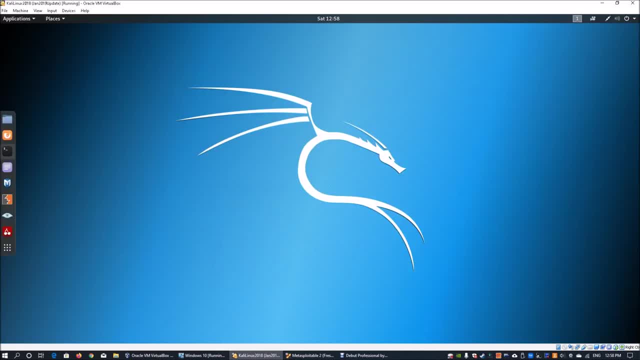 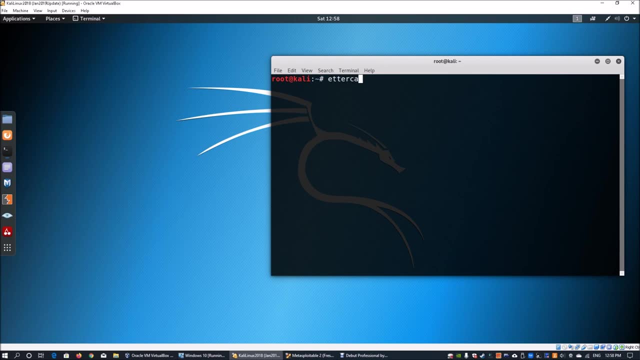 into Call Linux. So Call Linux. here is a virtual machine and we can open up terminal. So from here on we can zoom in a little so it's easier for you to see, and we can launch Adacap. So once you, 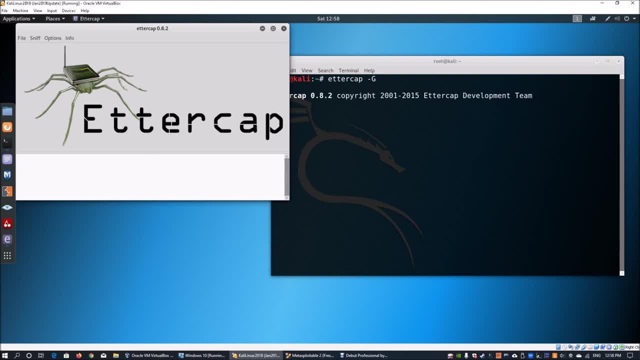 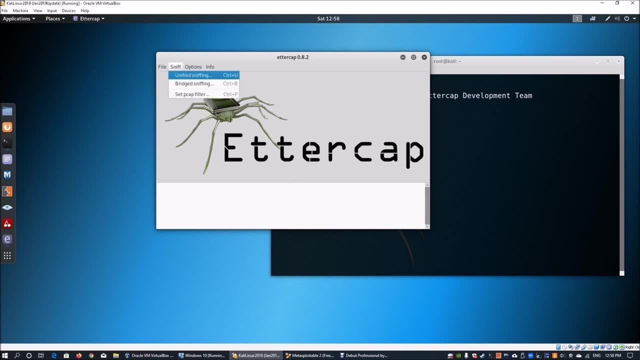 launch Adacap-G, it will boot up the user or graphical user interface of Adacap. So once you're in Adacap the first thing you go to is on the SNF. So when you go to SNF you go. 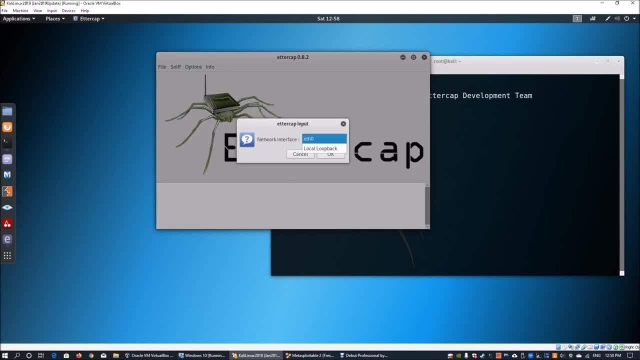 into Unified Sniffing and you indicate the network interface. So in this case, I only have ETH0 as well as a local loopback, So we are going to select ETH0.. So for your case, it could be a Wi-Fi, it could be a wireless, it could be any of those interfaces, So you have to choose them. 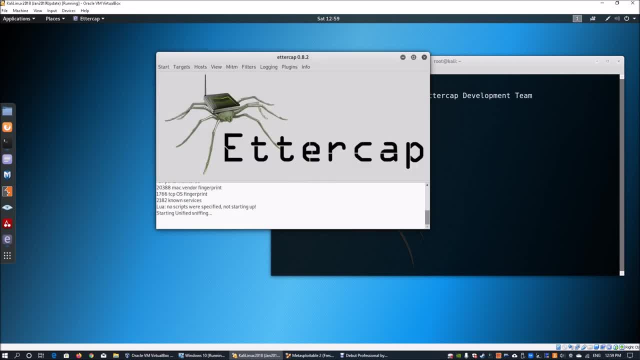 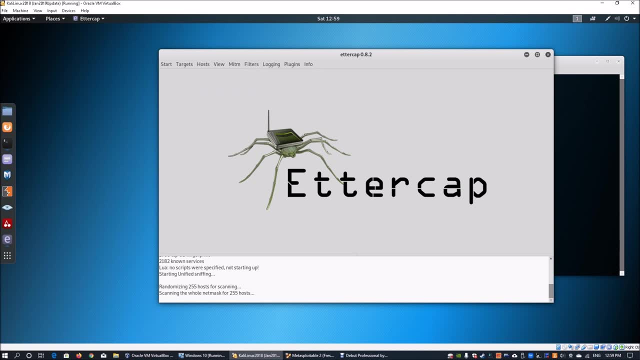 correctly. So go ahead and click OK and this would be able to start up the Unified Sniffing on Adacap. So, moving forward, the first thing we want to do is actually scan for hosts, So the entire subnetwork or the network mask, and tell you where are all the hosts. So if you go in to 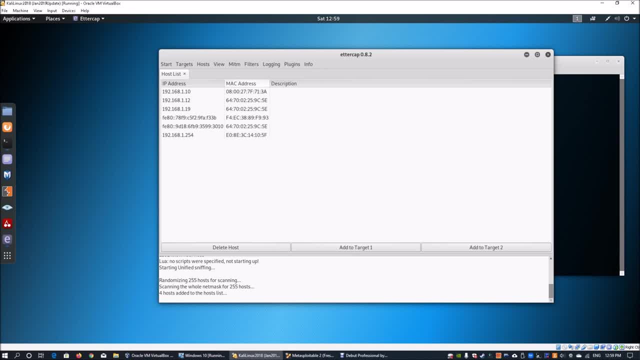 the host list. here we can see all the hosts within your subnetwork. So here, as mentioned earlier, we got a couple of IP addresses that we are targeting. So one is the 192.168.1.10, and we're going to add this as target one. And number two, we're going to go to 192.168.1.19,. 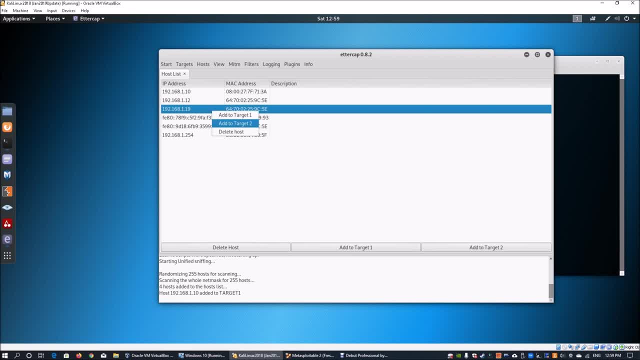 and we're going to target this as target number two. So we're going to add this to item two And once you've done that, you can go into the targets and you can look at the current targets. So from here you can see what are the targeting questions And, of course, 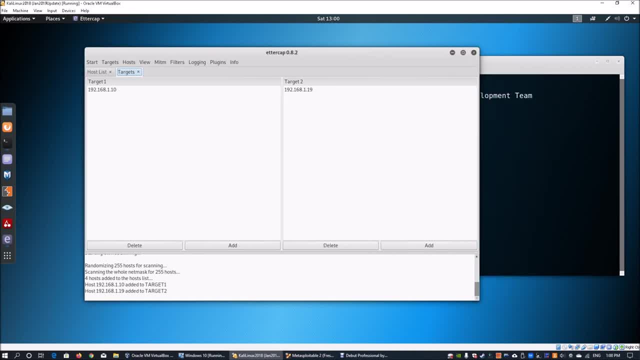 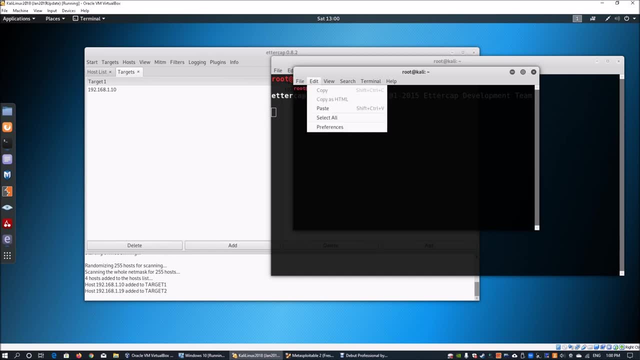 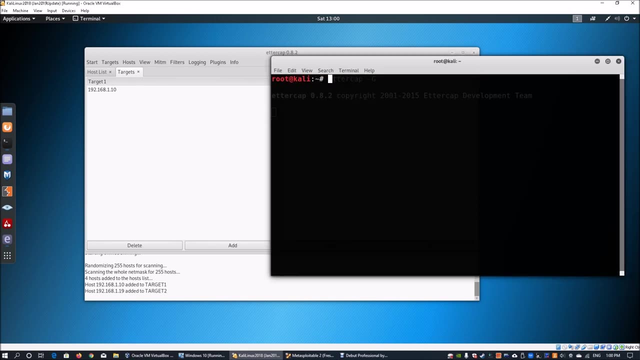 you can begin your ARP spoofing. However, before we go there, I'm going to launch a new window terminal, And on a new window terminal because we want to be able to capture all this traffic with Wireshark. so we are going to change some configuration within Linux. So the first thing, 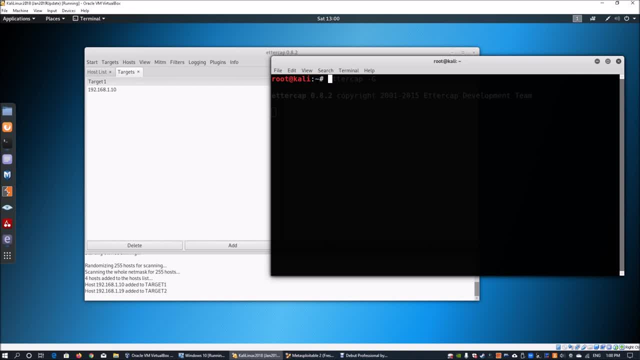 we want to do is we are going to change a way how we are looking into the traffic. So what we are going to do is we can enter or you can go into cat slash, broc slash, sys slash, net slash, ipv4 slash, ip underscore. 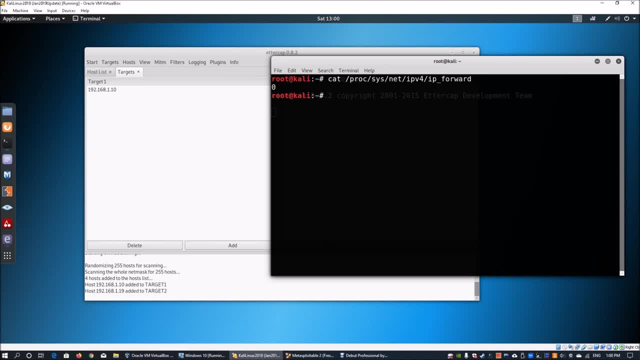 forward And then if you hit enter, you can see that the default value is zero. Because we want to start capturing, we have to change this to one. So we put echo one and we are going to enter that IPv4, followed by IP underscore, forward, And then you hit enter on that. 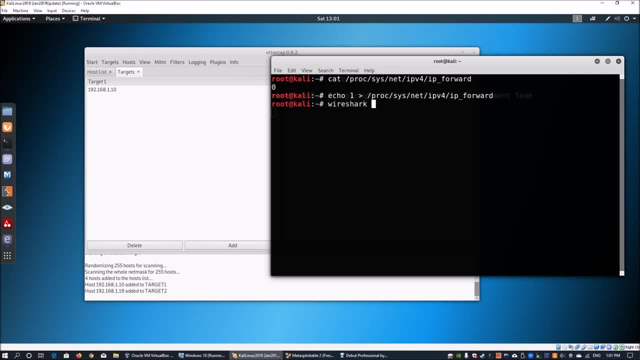 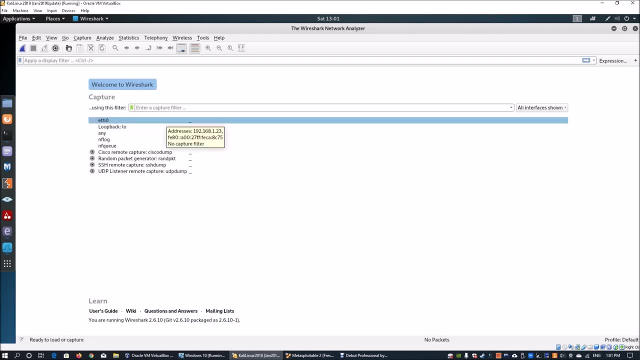 So once we do that, we have changed the configuration and we can launch Wireshark together with Adacap. So once we have Wireshark launched, we are going to capture all those traffic on ETH0.. So double click on it, it starts to capture. And now what we are going to do? 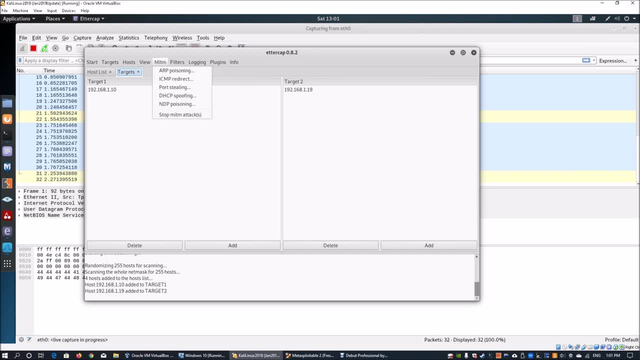 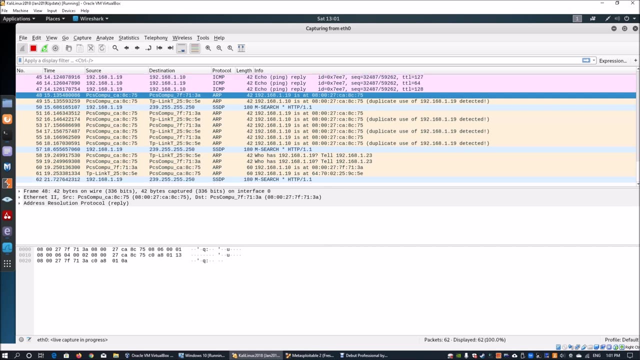 we go to Adacap and we go into the MITM, which is Man Intermediate Attack, We click ARP- ARP Poisoning- and we click Sneef- Remove Connections and click OK. So once you do that, on the backdrop of this you can see a lot of ARP information is being sent out into the